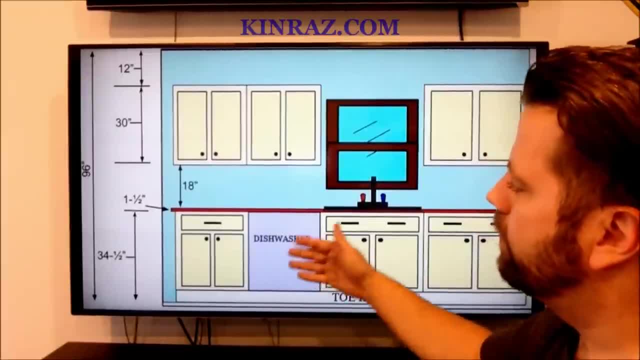 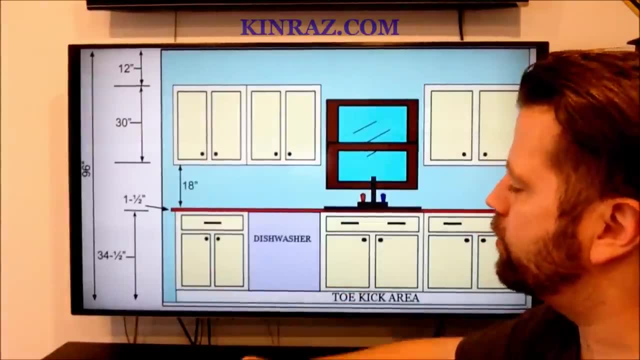 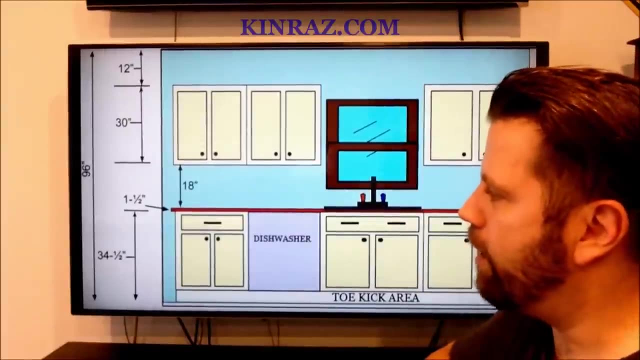 to set on that finished floor when they are installed. So, as far as sizes go, 34 and a half inches is your basic standard size for a kitchen base cabinet. Then, up above that, you have your countertop. Now, most of the time your countertops will be one and a half inches thick. That includes 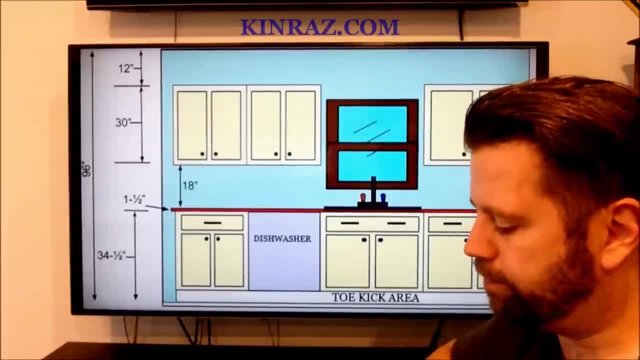 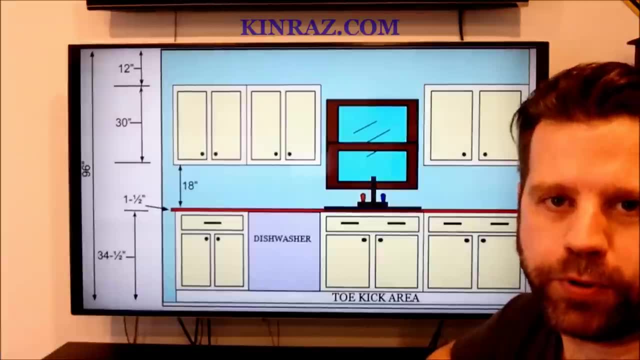 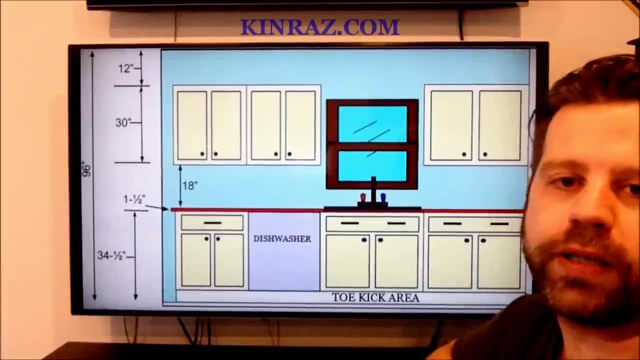 your laminate tops- That includes your solid surface tops- will be one and a half inches thick. If you did go with a hardwood, maple, butcher block countertop, that would also be one and a half inches thick. Some of the tops that will vary from that will be stone tops- Usually those thicknesses. 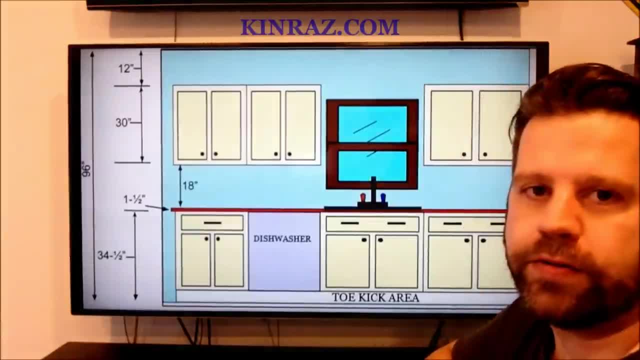 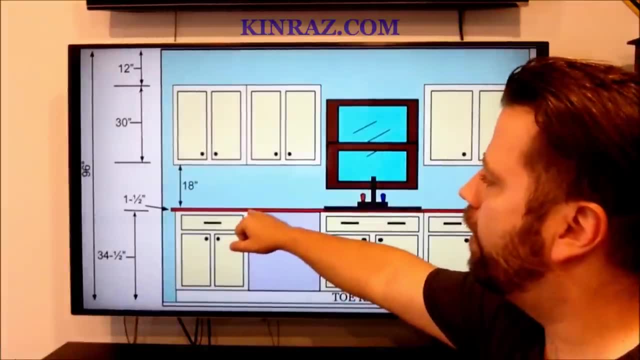 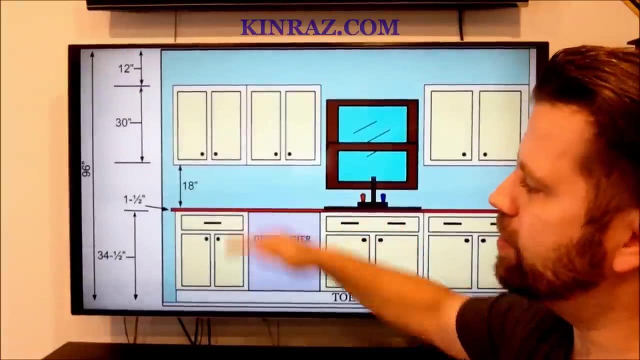 are rated in centimeters. Three centimeters is one and a quarter inches thick. Two centimeters is three quarter inches thick, So that can change Here as far as the thickness goes, But in general terms your countertop finishes out at 36 inches. 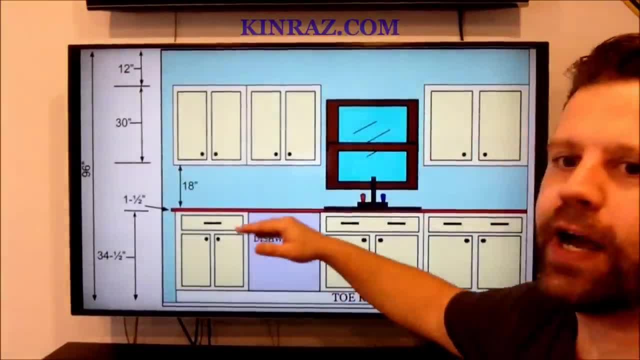 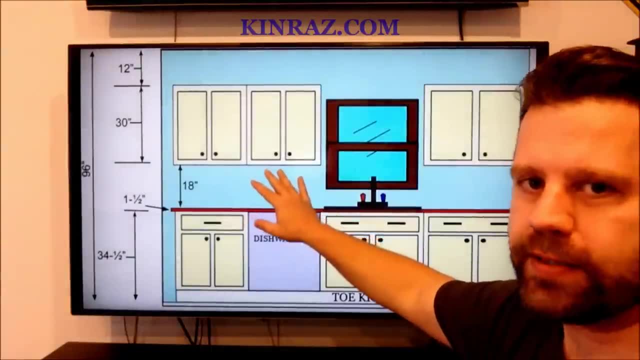 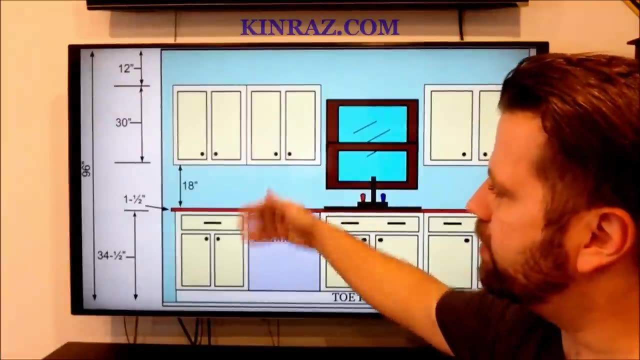 above the finished floor. Now, up above your countertop, you have your backsplash space. Now, most of the time, people will run ceramic tile here and put the ceramic tile on this. So the 18 inch space is a good standard to go with. 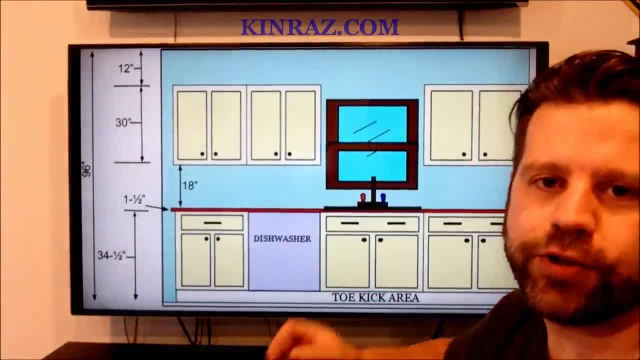 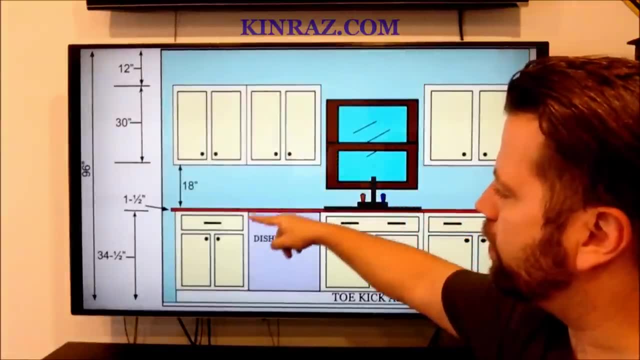 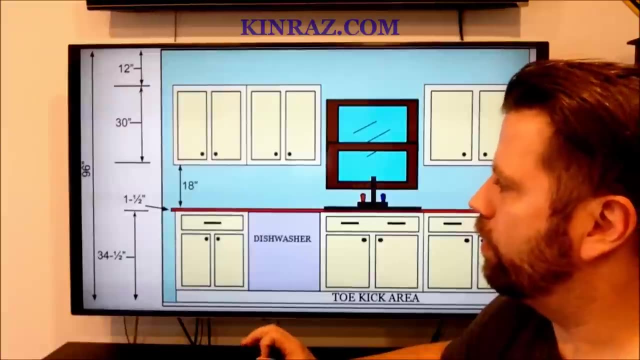 However, some kitchens have a shorter cook in the family. Now it is acceptable to lower these kitchen wall cabinets down to where you only have a 15 inch space instead of an 18 inch space. You never really want to go lower than 15 inches on the space in between. 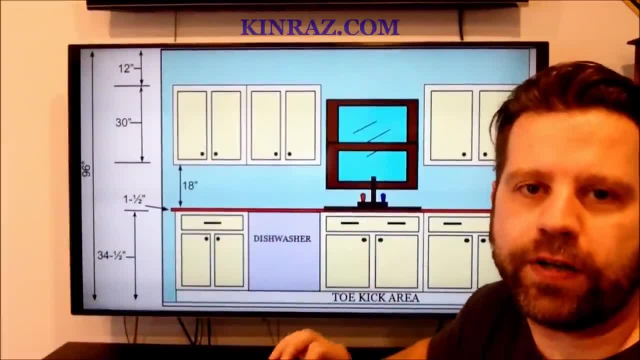 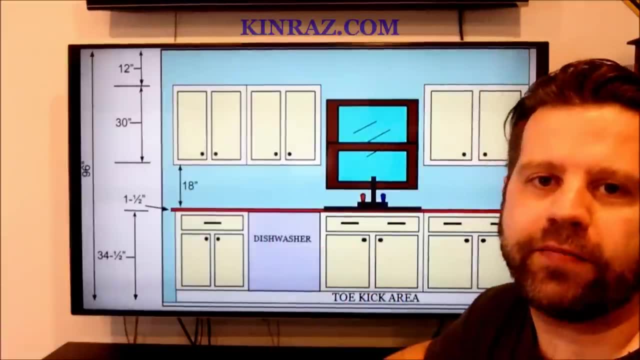 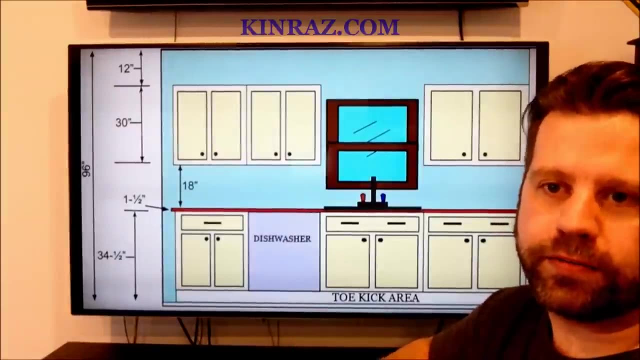 your countertop and your wall cabinets. Here's why, If you did a 15 inch space on your kitchen remodel- Any shorter than that- you're going to have a difficult time getting your coffee pots in there, your mixers, your blenders, some taller kitchen appliances. 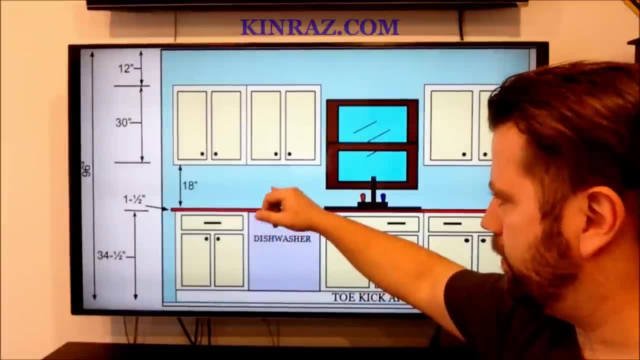 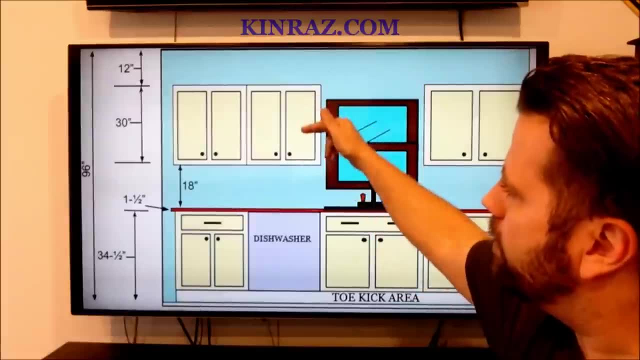 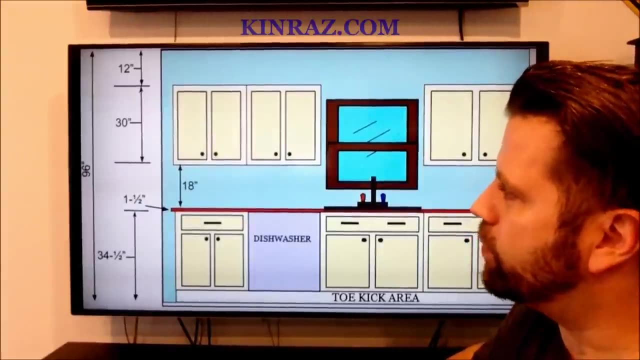 That can be an issue, So remember to always keep at least a 15-inch space, and preferably an 18.. And then, of course, up above that, we have a standard-sized wall cabinet. Those are generally 30 inches tall. Now they do sell them taller.